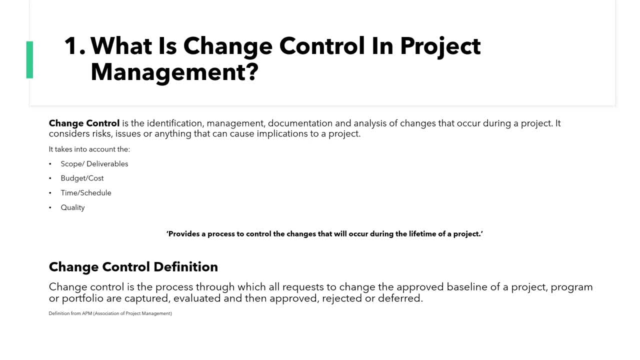 deliverables, the project budget or cost, any time or schedule for the project and the quality as well. So, in other words, change control provides a process to control the changes that will occur during the lifetime of a project, and I've also taken in a definition from the APM. 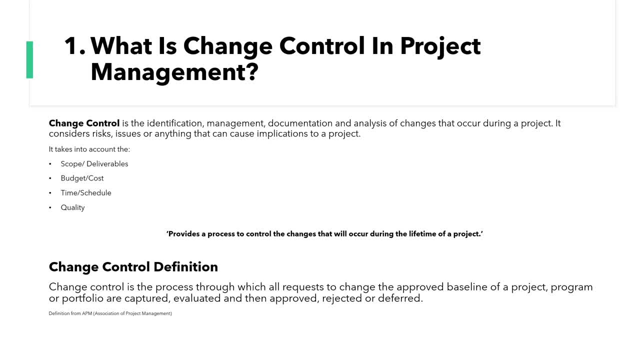 author. The proposed changes will take place during the entire project cycle. Change control is the process, so consider that term there. process Change control is the process through which all requests to change the approved baseline of a project programme or portfolio are captured. 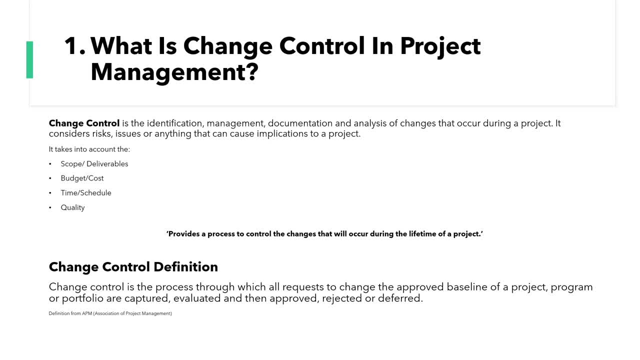 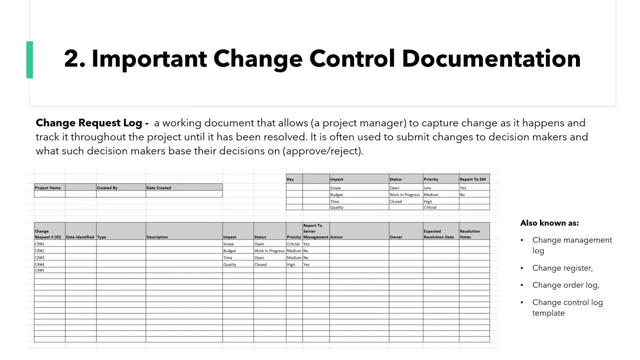 evaluated and then approved, rejected or deferred. So I'd like to introduce you to one of the key pieces of documentation for change control. Now I'm going to refer to here is the change request log, which is how it's typically referred to, but it is also known as a. 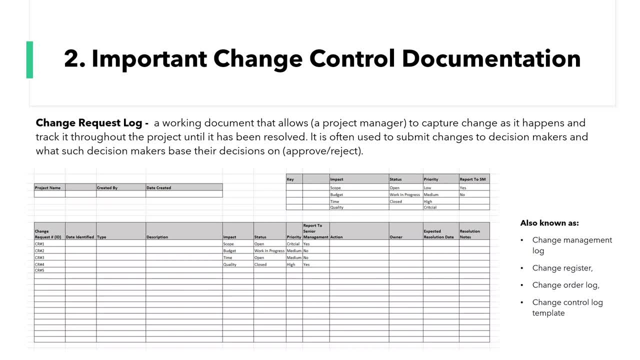 change management log, a change register, a changed order log or change control log template. so if you see those terms used, do consider that they. they are all the same thing. so this is a template that i've pulled together. i've put a link in the description below if you wanted to get access. 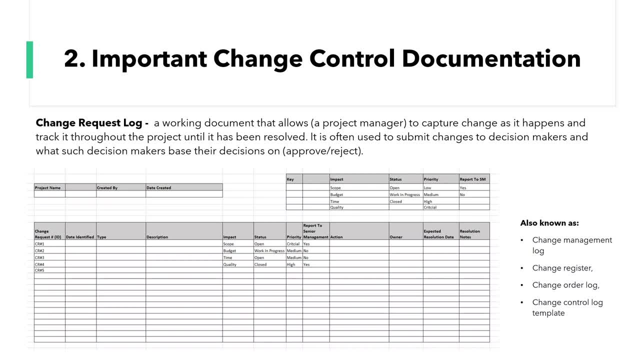 to this template. perhaps it will save you having to build one from your own it's it's all kind of pre-formatted, so you can just pick it up and start using it should you need one. but this one i'm trying to show you here is essentially what a typical change request log contains. 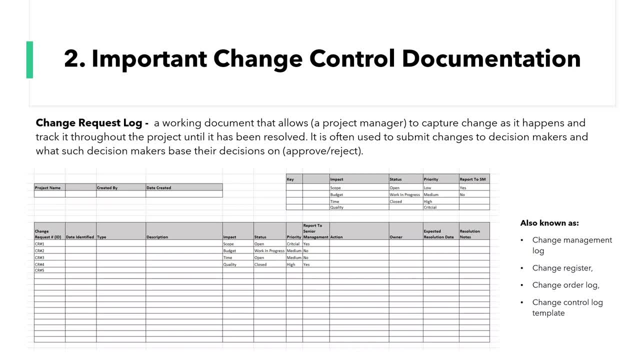 now consider that the change request log is a working document that allows a project manager to capture change as it occurs and then track it throughout the project until it has been resolved. so it is often used to then submit change these, these potential changes, to key decision makers and they will then use this information to make their decisions. so whether 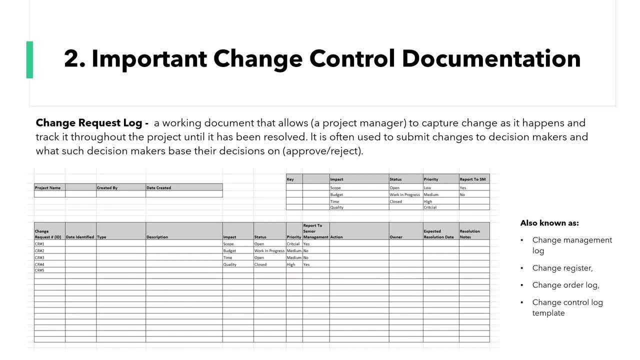 that's an approve, reject or even defer. so if we look here at this change request log in the far left we've got a change request id and that's obviously just used as a reference. the date identified is an important piece of data to collect the type. now that can be something like: 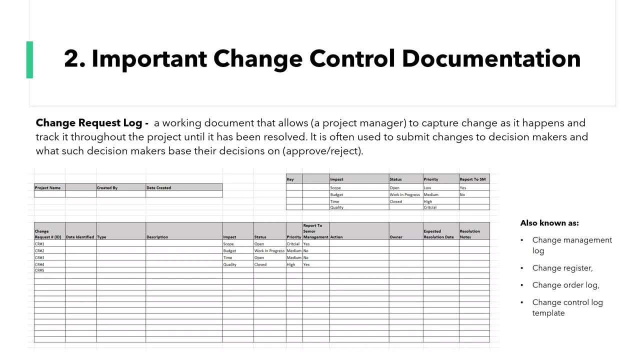 it could be due to resource. that could be resources. it could be something like a product. you get the idea. a description gives an i an overview of what the change will be. we've got an impact. so what? what area of of the project is it kind of impacting? is it the scope, the budget, the 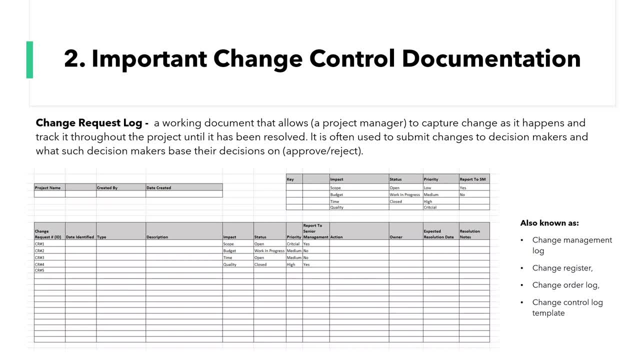 time or the quality, those um features that kind of previously discussed in the former slide. we've got a status. so you know what's happened to the to the change request: is it still open? is it work in progress? is it closed? a priority, so that helps to submit the right change requests at the right time. 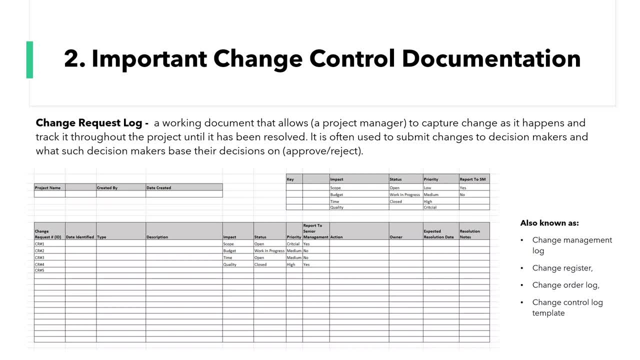 so you've got the change request. you've got the change request. so you've got the change request and you've got a report to senior management. so this is a yes- no flag that i've put in here. so that's whether it needs to go up the chain. so if you wanted to submit a change request and 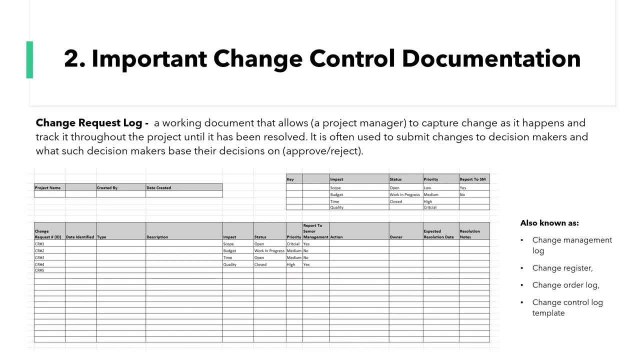 you could put yes in this kind of column: action, so that's what's actually being implemented for the change request. an owner- so that could be your yourself as the project manager or someone else within the project team. an expected resolution date and and a field to enter any resolution notes. 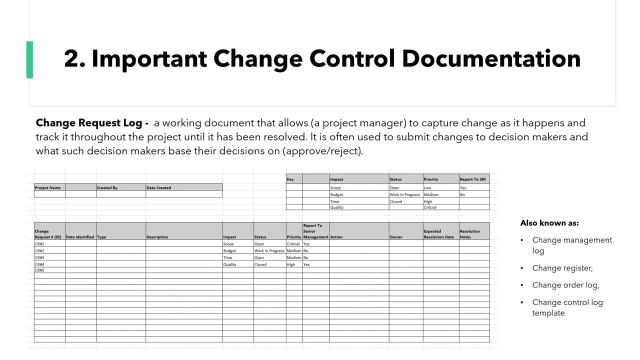 now consider. this is typical for a change request log, but you may look at different templates and they may contain different columns or variations of these, so just bear that in mind. when it comes to project management documentation, you will find that there is variance, so don't be too disheartened. 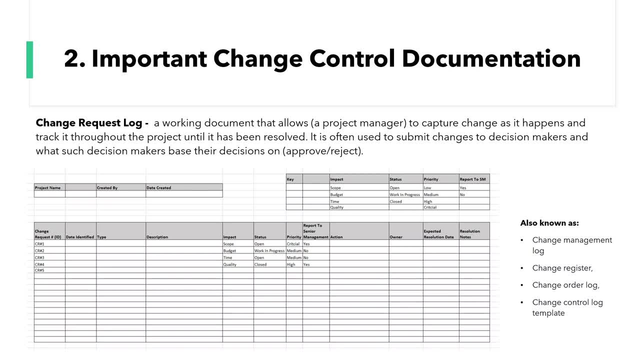 if you don't have everything that every change or project management template has. the key and important thing to remember here is that you have the key pieces of data and the data that will actually help you in your organization. it's also not a good idea to have too many. 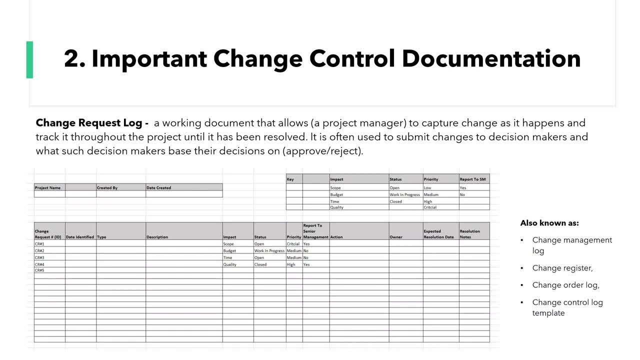 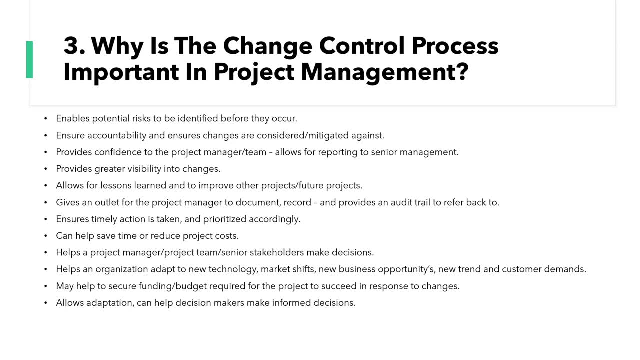 columns or too much data you want. the essentials are set, basically. so why is change, the change control process, important? well, it enables potential risks to be identified before they occur. it ensures accountability and ensures changes are considered and perhaps even might get mitigated against. it will provide confidence to the project manager or team and it allows for the reporting to 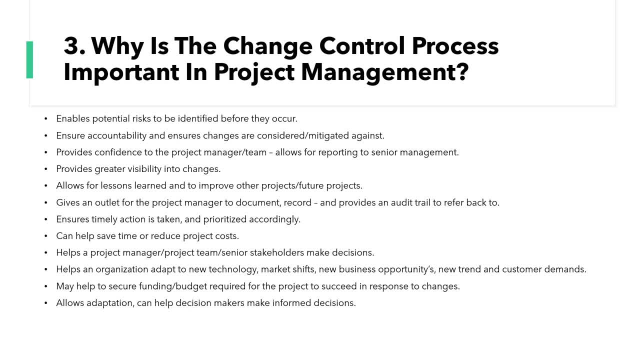 senior management so that they are kept in the loop and are fully aware of what's going on. it provides greater visibility into any changes, it allows for lessons learned and it also allows for other projects or future projects to be kind of improved upon and kind of more insight into what's going on. it gives an outlet for the project manager to document and 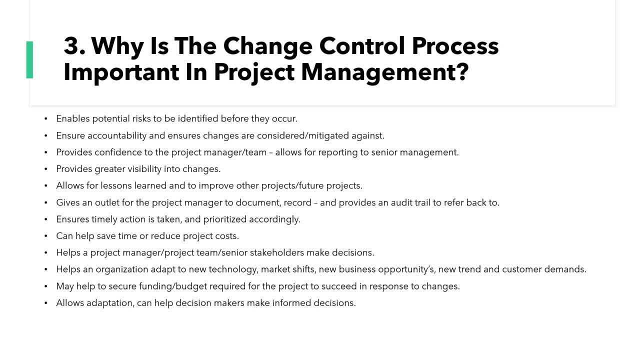 record. so in that respect it provides an audit trail to refer back to. it also ensures the timely action and prioritization as well against particular changes or change requests. it can help save time or reduce project costs or ensure that a project meets its deadlines. it helps project managers. 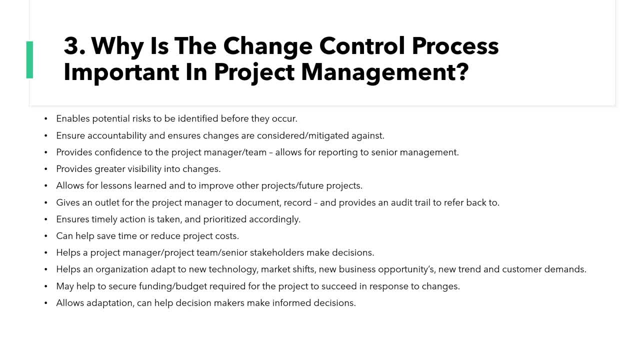 team members and even senior stakeholders make decisions. that's really, really important here. it also helps an organization to adapt to new technology, shifts in the market, new business opportunities, upcoming trends or even changes to customer demand, either in advance or expectations. it may also help a project manager to secure necessary funding or 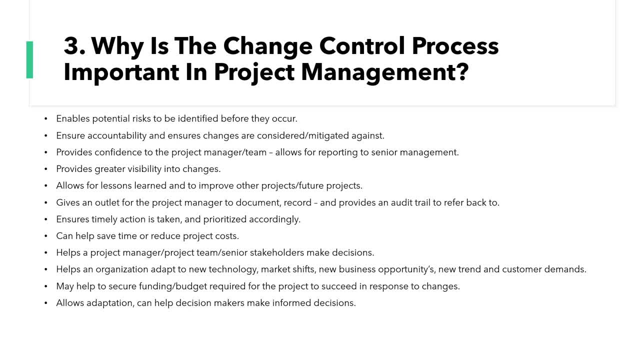 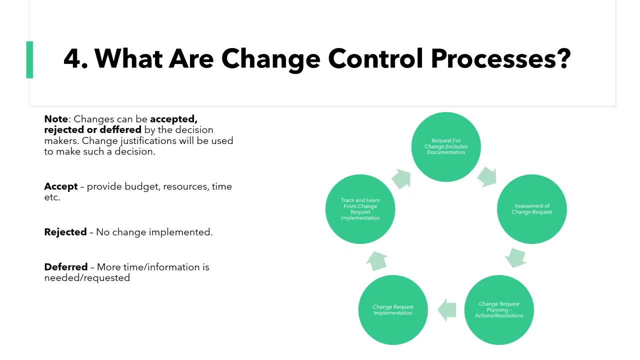 budget for the project to succeed in response to these changes. in a nutshell, change. the Change Control process allows adaptation and it can help everybody make better informed decisions. so I've provided you here with a quick overview of what a change control process is, or the processes look like. 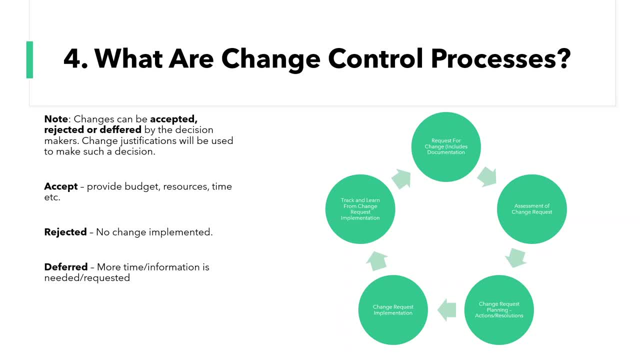 processes, or the processes look like On the left hand side. I just wanted to make notes that when change requests are submitted to decision makers, they will then have the option to either accept, reject or defer them, And any justifications put forward by the project manager will be taken into. 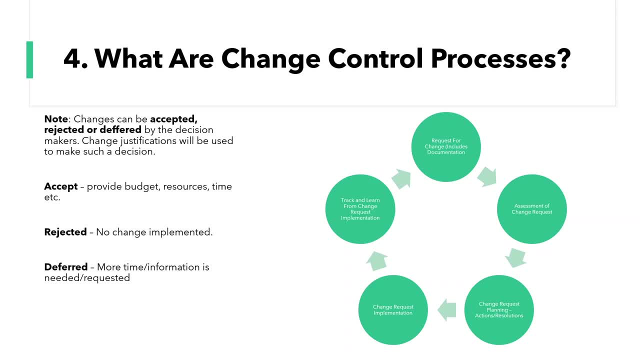 consideration to make such a decision. So if a change request is accepted, it may be that the project manager or the project team is provided with additional budget, maybe even more resources, or maybe there'll be a change to the project scopes and they may be given more time to complete. 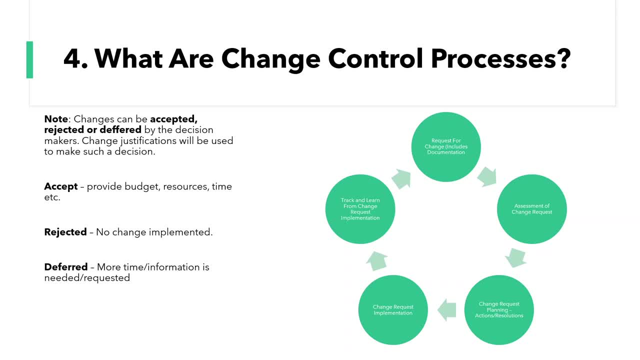 the project. If the change request is rejected, then no change is implemented And while it may be kind of it caused some issues, the decision makers have made the decision that there's no need to move forward with the change request for whatever reason For deferred. it may be that 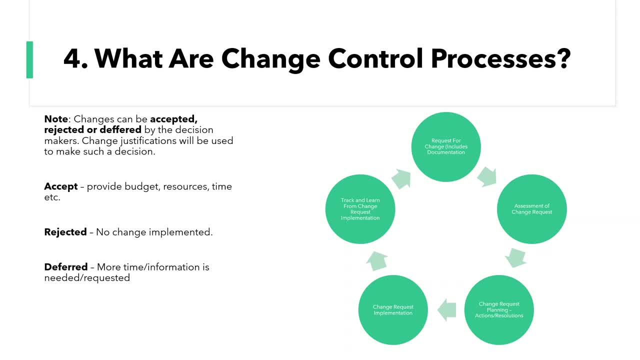 more time or more information is needed or required or even requested in order for the change request to be kind of reviewed again. So in the middle, on the right hand side, I should say here, I've got an overview of the process, starting at the top. so the request for change. 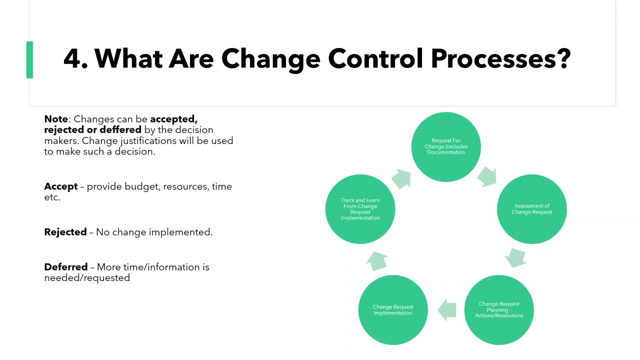 is the first part of the process and that's when it's kind of documented in the change request log. Next you have the assessment of the change request. so that would make sure that everything's kind of considered The change request. planning would then take place and that would. 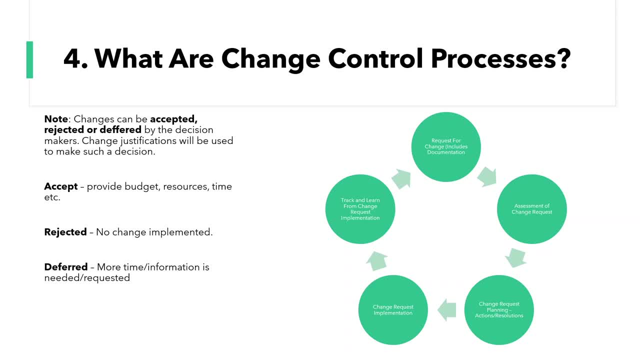 include any actions or resolutions that need to be put into place for said change request. Then, if it is accepted or approved, then the implementation would occur. I should have put in this little one here that if it's rejected or deferred it would then kind of stop there. so do consider that. but 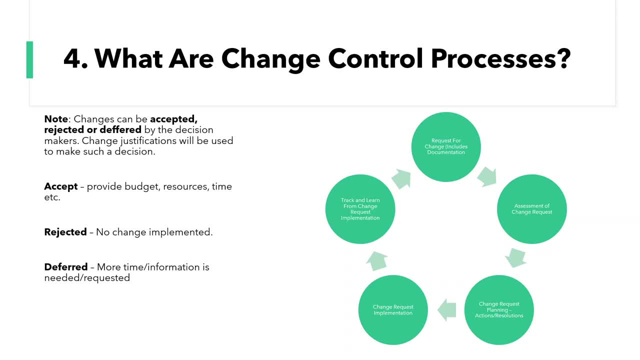 if it is accepted, the change request would be implemented. and then, off of the back of that- if it is accepted- then the change request would be tracked and the implementation would be reviewed So that the organisation or the project manager or team could learn from such a request, if it is. 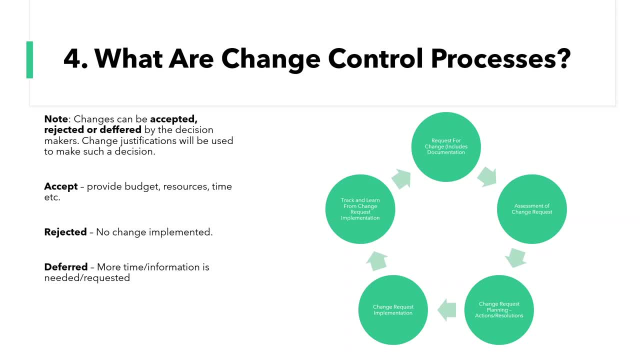 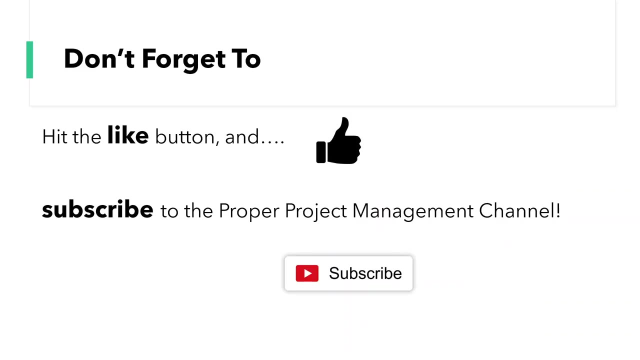 rejected or deferred, then it literally stops there, and unless additional justification is provided by the project manager, then the change request is: it stops. That's it, it's over, it's not, it's not being implemented. So I hope this video is useful. if it was, please do hit the like button. 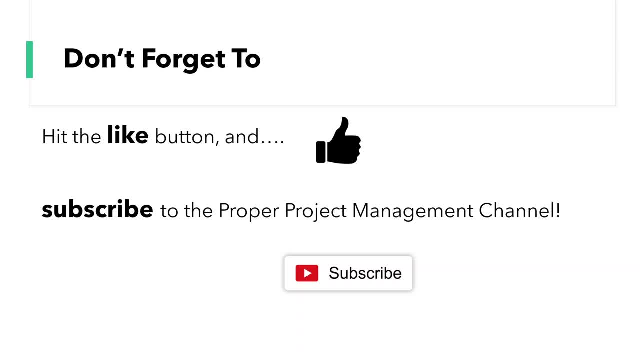 that tells me I should continue making videos like this and if you haven't already, please consider subscribing to my channel. If you head over to my channel, I've got a playlist on. I've got various different playlists on project management, training, whether it's concepts like change control. I've got playlists on creating. 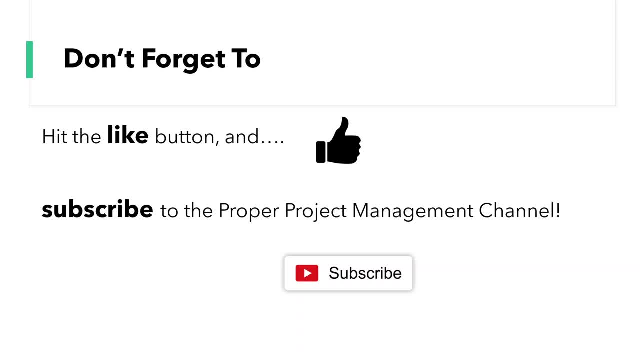 project management templates and artefacts if you need to create them, and I also have videos on project management softwares, such as the likes of whether it's excel using excel or you're using more of a paid tool. so if you're using a paid tool, you're using a paid tool. so if you're using a paid tool, 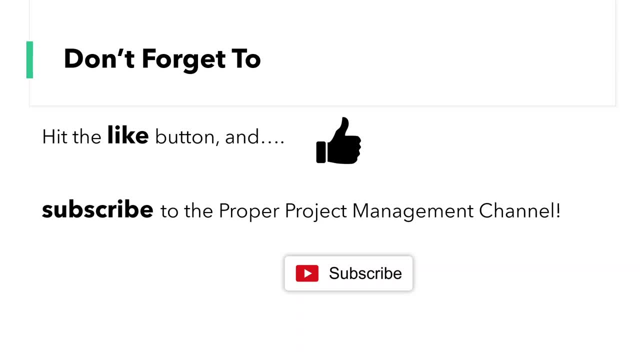 such as smartsheet or asana. there's videos on the on them too. so, with all that said, I hope you have an excellent day.